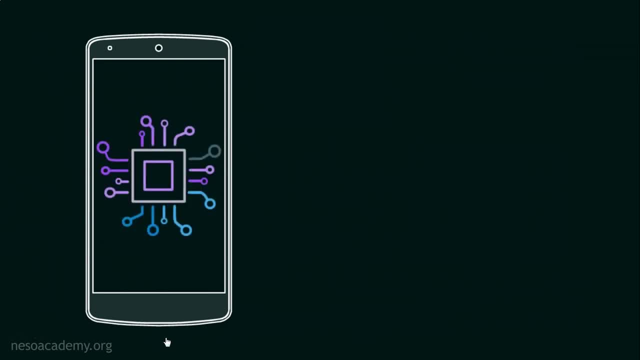 today we have gigahertz processors, even in our smartphones. Suppose we have 2 gigahertz processor, This means the frequency is 2 gigahertz, Hence time is 1 upon frequency, that is, 1 by 2 into 10 to the power 9.. 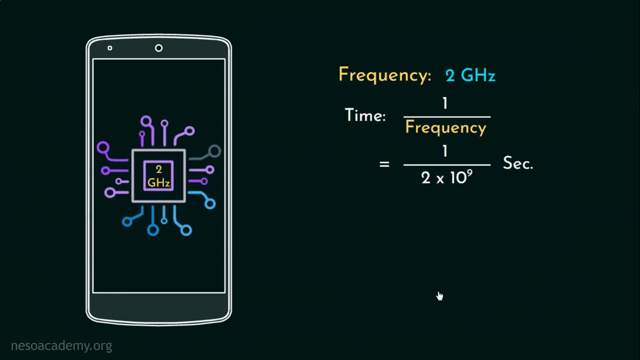 Now, how did I get this 10 to the power 9?? Let's have a chart, shall we? We know 1 kilo unit equals to 1000 units, hence 10 cube units. Therefore, 1 mega unit is 1000 kilo units, and thus 10 to the power 6 units. And finally, 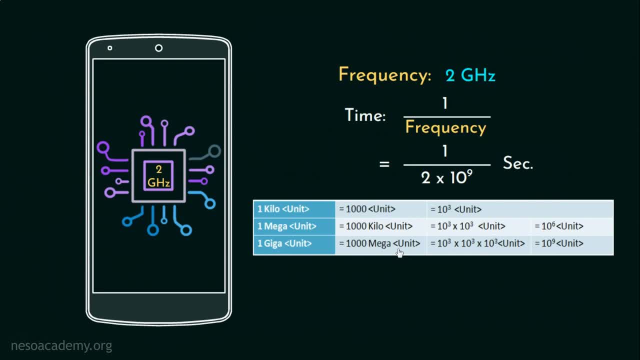 1 giga units is 1000 mega units, and thus 10 to the power, 9 units. Now coming back to our initial illustration: 1 upon 2 into 10 to the power. 9 seconds equals to 1 by 2 into 10 to the power. 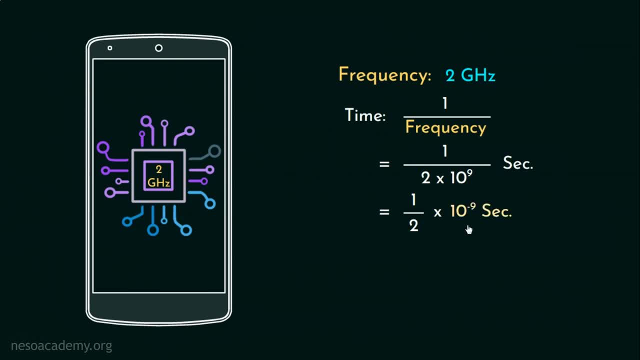 minus 9 seconds and 10 to the power minus 9 seconds is 1 nanosecond. Therefore, in half a nanosecond our processor can perform a single task. So to conclude, the CPU is fast, not only fast, real fast. and keeping up with this kind of speed is tough because if our memory device is way slower, 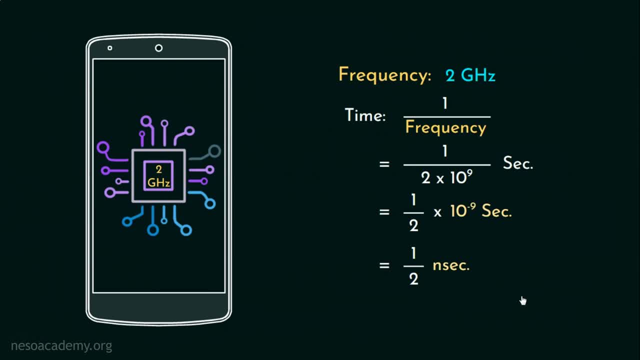 than the CPU, then the CPU will remain idle for the most of the time and we won't have an efficient machine. Also, not only the speed, the size and the cost are considered too when it comes to memory. That's why we have various memory devices associated to our computer. Computer designers. 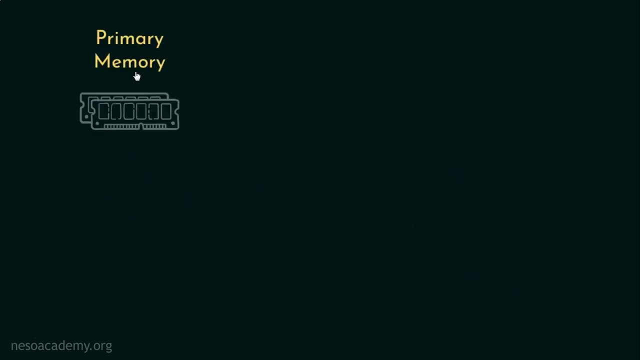 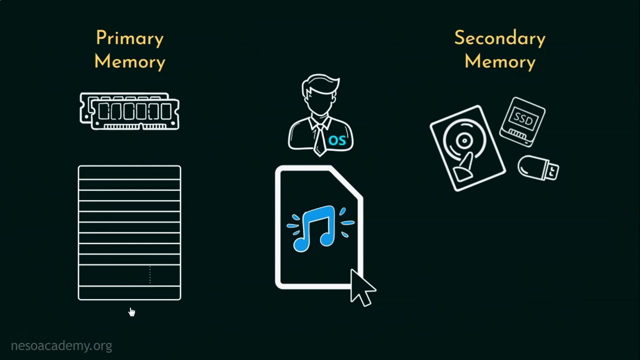 term the memory to perform immediately. The memory which is used as a more permanent storage is known as secondary memory. When we play an audio file, our system manager, that is, the operating system, manages the space within the primary memory to perform the instructions, which is understanding the mouse click, opening up the. 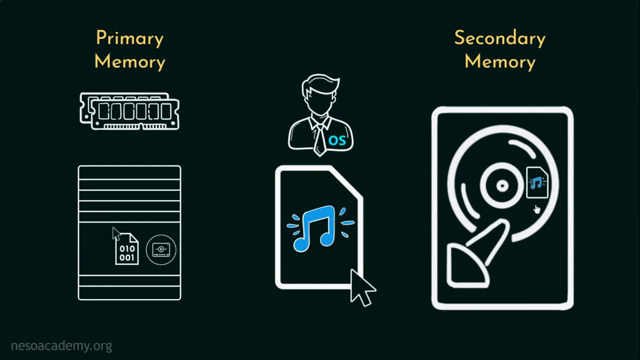 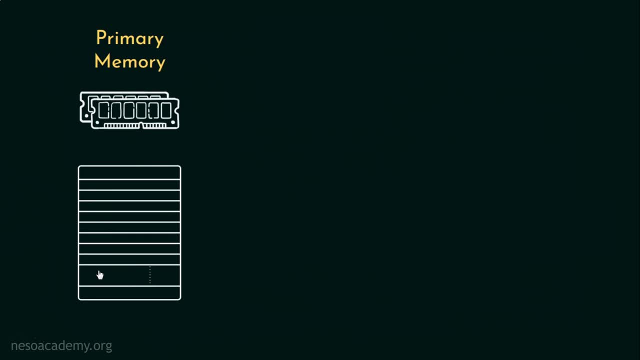 default application for playing the file after bringing it from the secondary storage into the primary memory. Now, as because we need the execution of the instructions to be as quick as possible, the sales in the primary memory can be accessed in any order, and that's why the name random access memory or 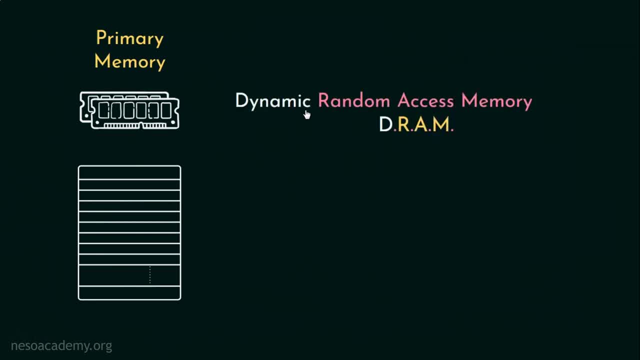 RAM. To be precise, it's actually dynamic RAM, because in each memory chip there is a transistor with which a capacitor is associated. The transistors can retain the binary bit as long as the associated capacitors have charge. So periodic recharge is a very important part of the 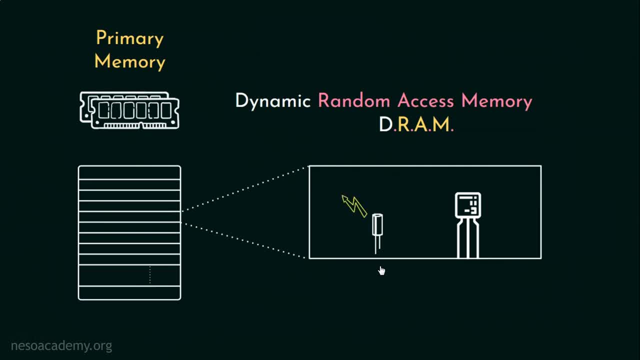 process. So we need to make sure that we have enough memory to be able to use it in any order, and that's why it's called dynamic. but it's still slow for the modern day processors, So we opt for another fast memory storage: the cache. Now, the cache is made up of static RAM which doesn't have any capacitors. 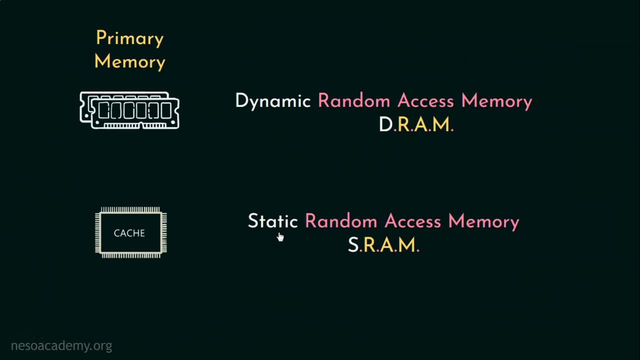 but they are very costly. in comparison to the main or primary memory, However, cache happens to be the fastest memory storage among all others. Anyway, all these, be that cache or main memory, are volatile. That means they can only retain the data in them until the power is off. 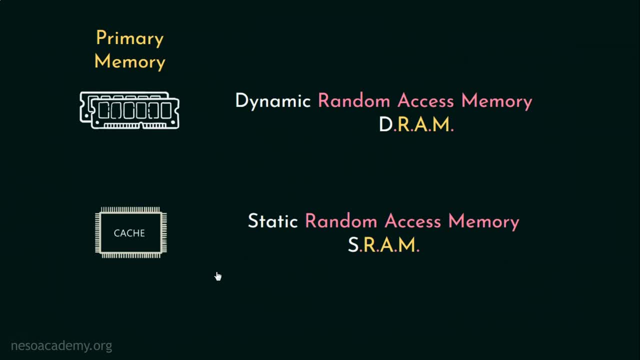 Therefore, to store the data more permanently, we opt for the next type of memory storage: The secondary memory. Now, secondary memories are slower than the main memory, yet they can retain data permanently. That is, the data inside them are still there, even if the power is off. They are. 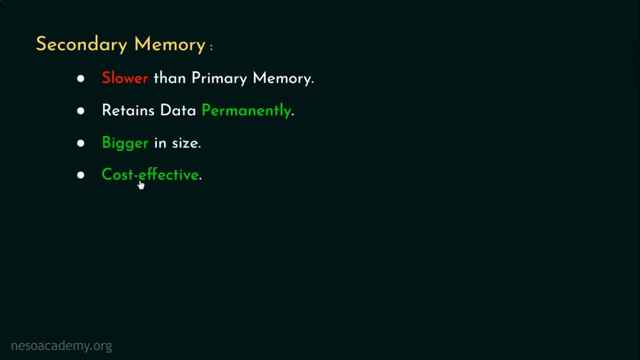 larger in terms of capacity. Also, they are cheaper than the main memory. We will definitely get into the detailed study of various types of secondary memories in our due course, But for the time being, I would like to take an example of one of the most popular secondary storage devices, that is, the hard disk drive, to explain. 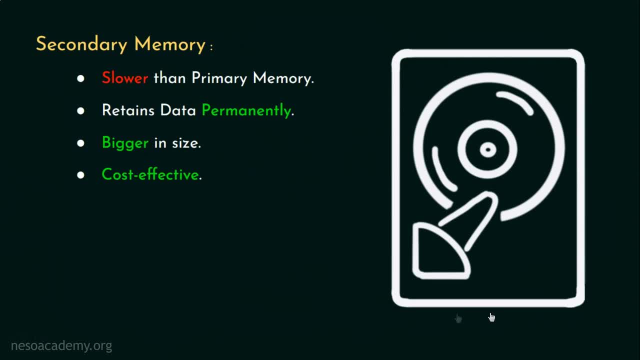 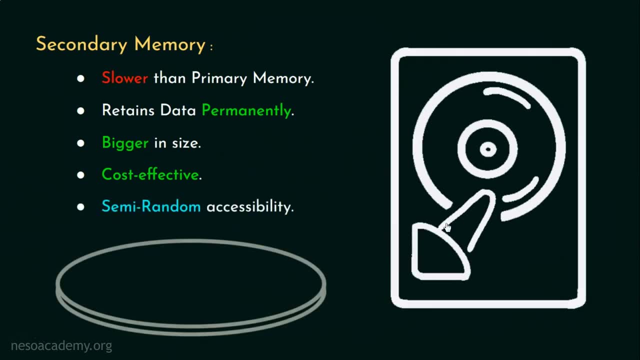 one of the reasons why these are slower compared to the main memory. For a hard disk drive, the axis is semi-random. Now why is so? Because, using this read write head, we can randomly get the data from any of these tracks, but from there getting to the particular block where the data is stored. 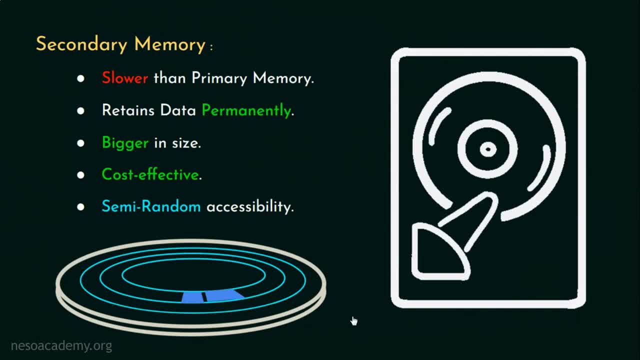 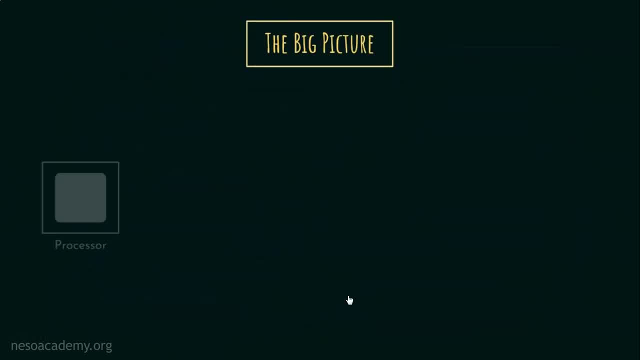 requires sequential movement, So the time to access any data in the hard disk drive becomes longer, naturally. Now let me show you the big picture. We have the processor and it has got its registers, but these are not capable of storing large amount of data. To be really honest, they can barely store